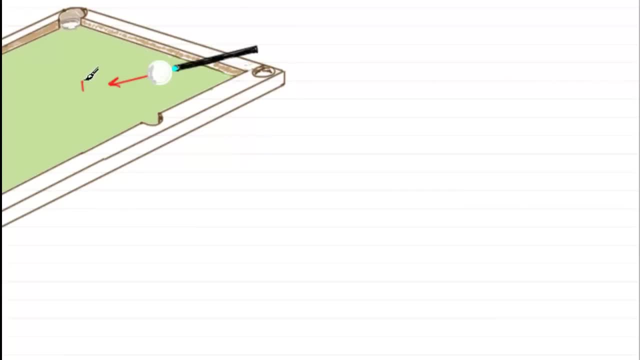 say, we illustrate it as a force F and we look at the acceleration produced, then there is a direct link between the force and the acceleration And that link was that the force was produced by the acceleration. So the force applied was proportional, was directly proportional to the 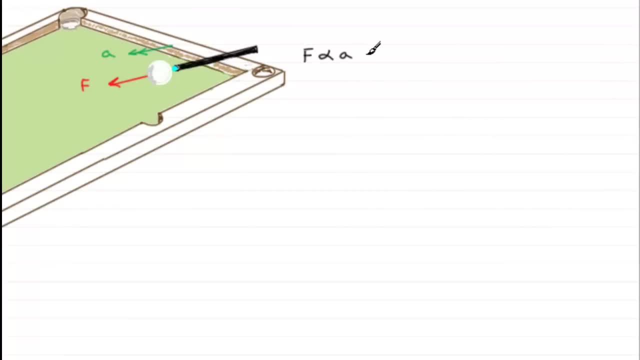 acceleration produced, And this led to the equation that that force F was equal to a constant multiplied by the acceleration, And that constant turned out to be the mass of the particle, M. So F equals MA, And this particular equation is known as Newton's second law. Let's just write that up here. 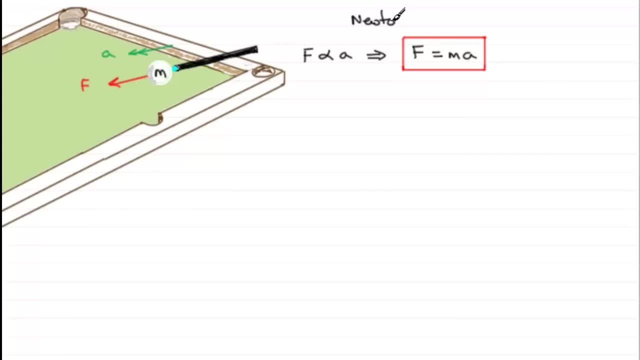 Newton's second law. Now you'll also see some people mention this equation as the equation of motion, So do learn it as that as well. So let's have a look at these units. The force here is measured in what is called Newtons. okay, 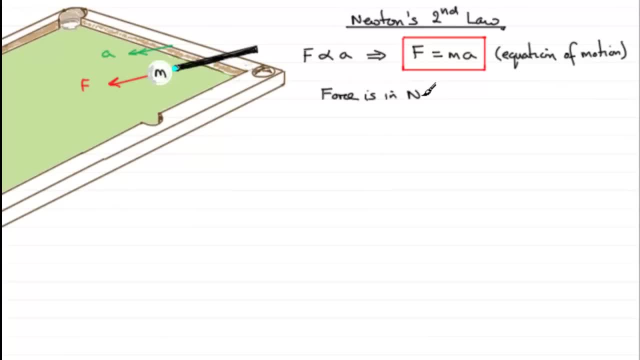 Force is in Newtons, And the standard symbol for a Newton is just simply an N: The mass is measured in kilograms. The mass is measured in kilograms, And the standard symbol for a Newton is just simply an N: The mass is measured in kilograms. 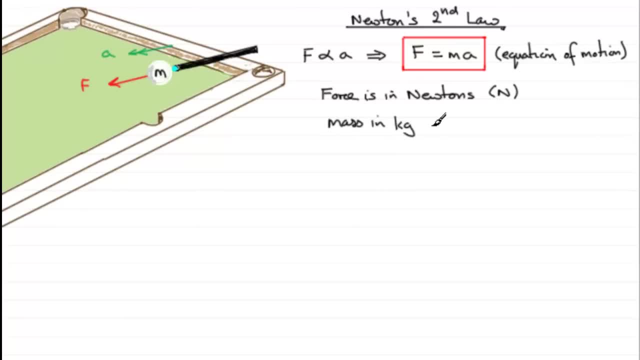 So do learn it as that as well. So just write that in in kilograms And the acceleration A. okay, that would be measured in meters per second, per second. Now we should look at some examples that use this equation: F equals MA. the equation of motion. 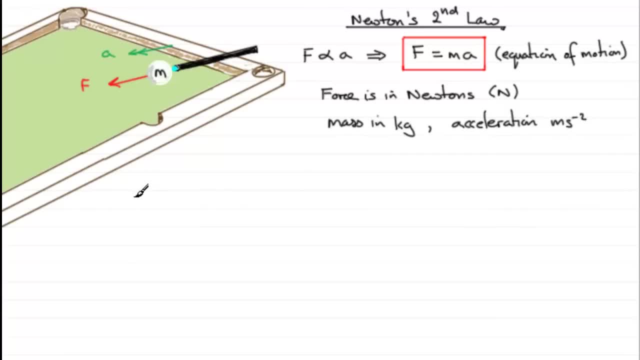 So suppose we had a particle, Let's say a particle of mass five kilograms- Let's just write the five kilograms inside- And to this particle we apply a force, say to the right of 10 Newtons, And this force is going to produce an acceleration in that direction, to the right. 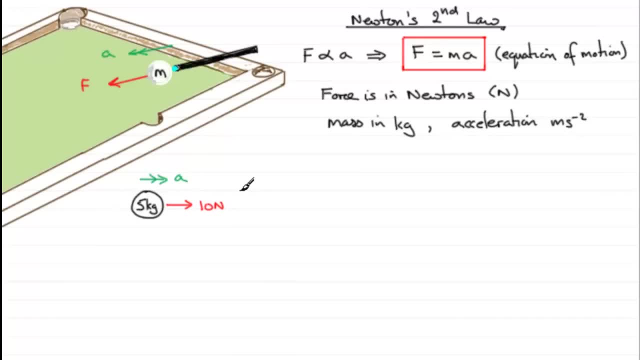 And we'll mark that in as A. Now, to apply F equals MA, the equation of motion. What we tend to do is write this: okay, R, which stands for resolving or applying Newton's second law, And we're showing that we're applying it to the right. okay, taking the right as positive. 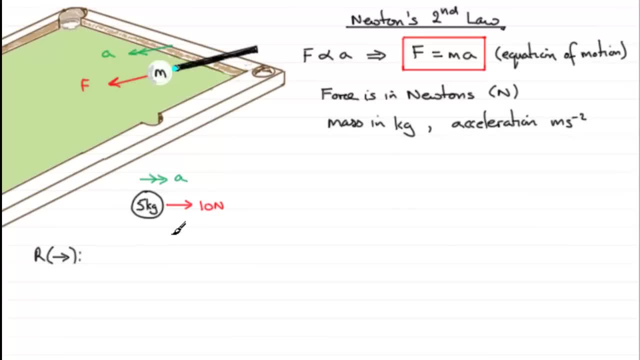 Remember force and acceleration of vector quantities. So we need to obey this positive rule. So we need to obey this positive rule. 10 Newtons acts to the right. okay, So it's going to be the force plus 10, or just simply 10.. 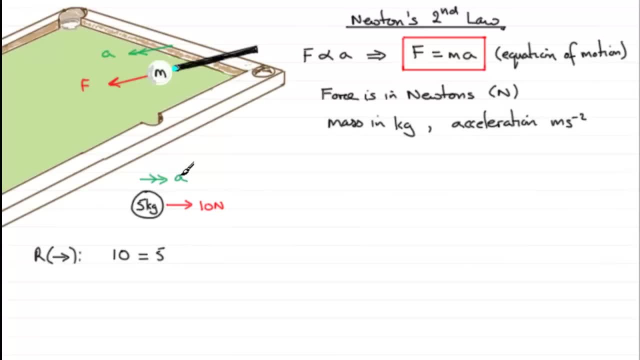 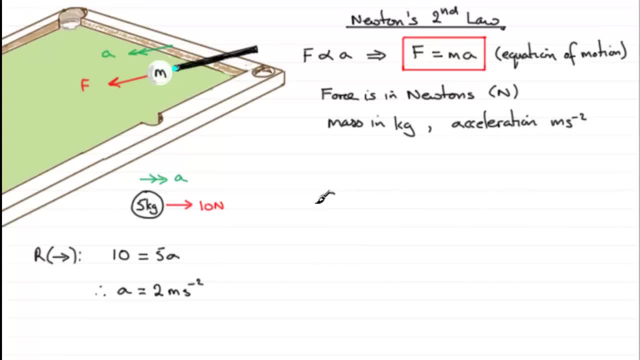 Okay Well, let's just look at this equation. Okay Well, let's just look at this equation. Let's just take another example again. We'll still stick with our 5 kilogram mass, But this time let's suppose we still got our 10 Newton force acting to the right. 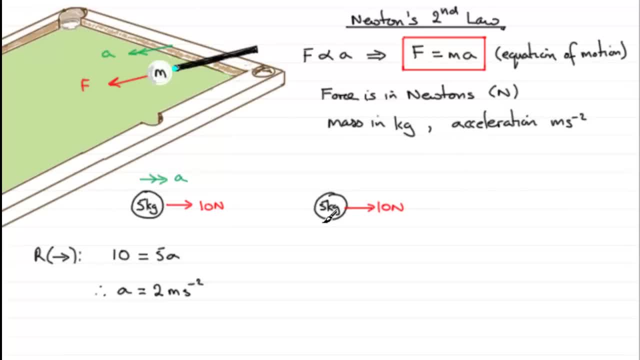 But maybe there's some resistance on our particle opposing this force to the right. Let's say it's a resistance, say, of 4 Newtons. Then what would the acceleration be this time? Well, we'll call it A again and we're going to resolve in the direction of motion. 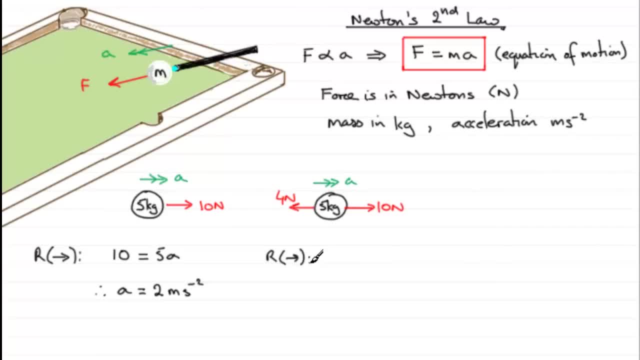 We'll resolve to the right, taking to the right as positive indicated by the arrow. So we're looking at the resultant force, F acting on this particle in this direction. So we've got 10, but the 4 newtons acts in the opposite direction, so it's going to be negative. 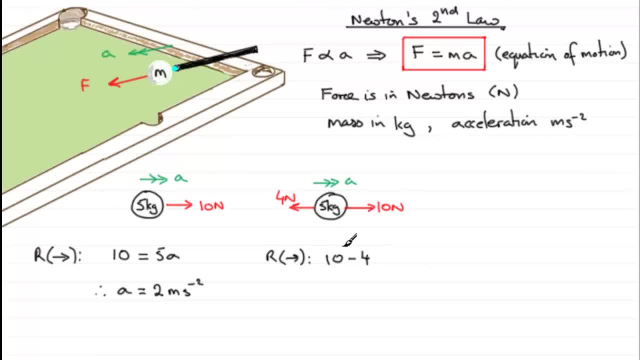 So it's going to be minus the 4.. So you can see we've got a resultant force of 6 newtons acting towards the right, And this is equal to the mass 5, multiplied by the new acceleration A. So what we've got here is 6 equals 5A. 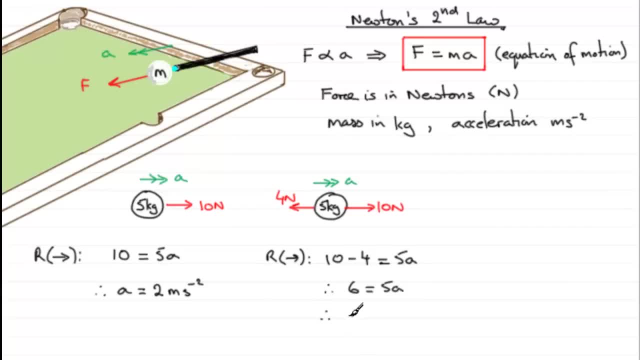 That's the new acceleration A. So what we've got here is 6 equals 5A, And dividing both sides by 5 gives us the acceleration is 6 fifths, or 1.2 metres per second per second. So you can see, once we've got this, resistance in the acceleration is reduced compared with what it was here. 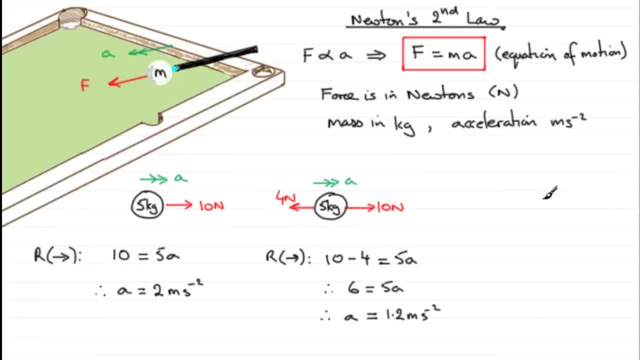 Now suppose we look at one more example. Again, we'll take our 5 kilogram mass, We'll have our 10 newton force acting to the right. But suppose we have a resistance, this time of 10 newtons. Then what's our acceleration going to be? 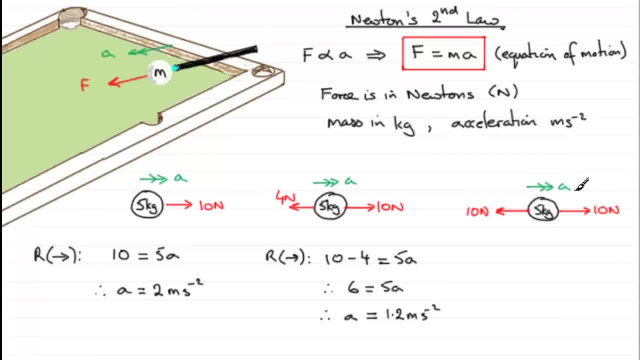 What's actually happening to this particle? Well, if we resolve, to the right, apply that equation of motion, Then what we've got here is a force acting to the right. So we've got a force of 10 newtons to the right minus 10 newtons to the left, a resultant of 0 newtons. 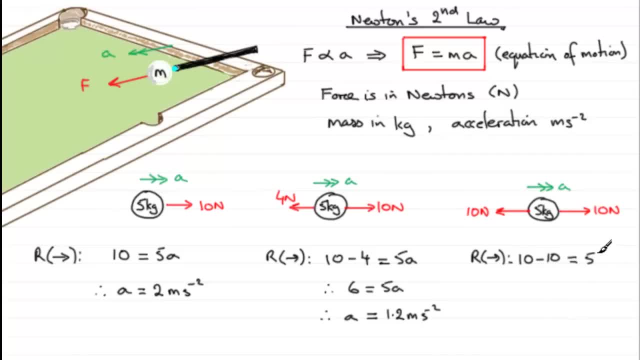 And this is equal to the mass 5, times the acceleration A, So we've got no resultant force and it equals 5A. And that would mean that the acceleration was equal to 0. 0 metres per second, per second. 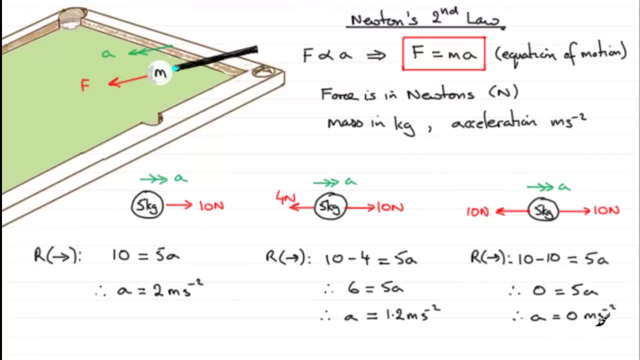 Now, when we have this, we can see that the acceleration was equal to 0 metres per second, per second. Now, when we have an acceleration that is 0, this can mean one of two things. It can mean that the particle is either in equilibrium, not moving. 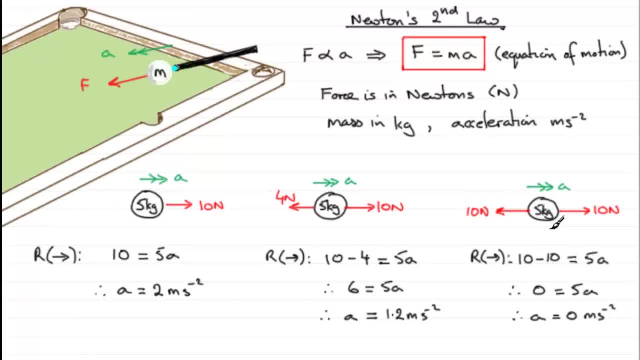 Or it's moving at a constant speed. Now, this is just a simple introductory tutorial on Newton's second law. In later videos I'll be exploring this equation a lot further. We'll be looking at forces inclined at angles to one another. We'll be looking at particles moving on inclined planes or connected by light inextensible strings passing over pulleys.